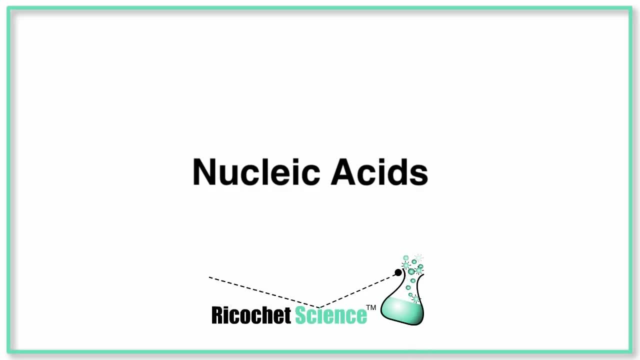 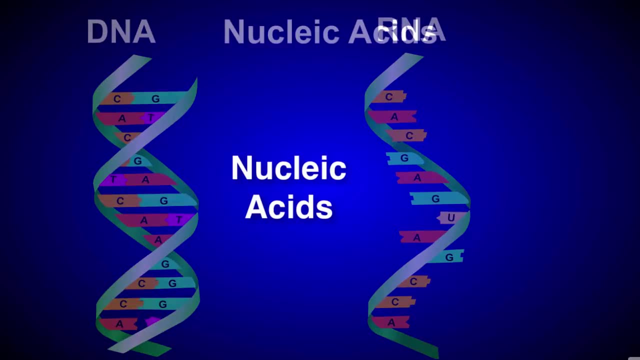 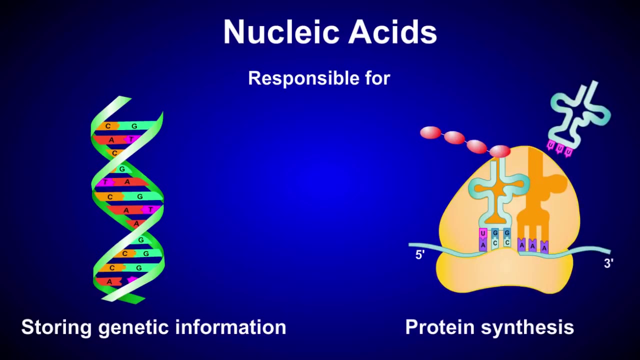 Nucleic acids are a class of biomolecules that are found in all living organisms and are responsible for the storage of genetic information. They are also responsible for protein synthesis. Nucleic acids are made up of monomers called nucleotides. 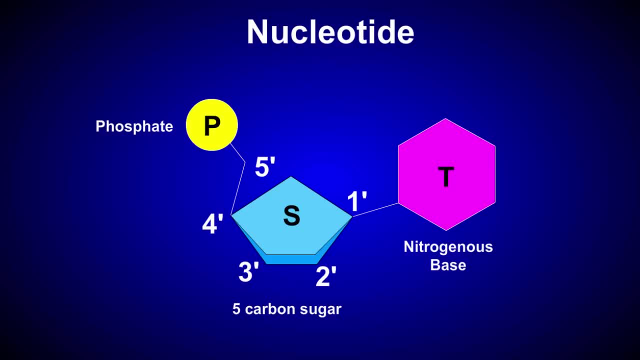 Nucleotides are made up of three components: a 5-carbon sugar, such as ribose, a phosphate functional group and a nitrogenous base. The 5-carbon sugar present in DNA is deoxyribose, and the four nitrogenous bases are adenine, guanine, cytosine and thymine. 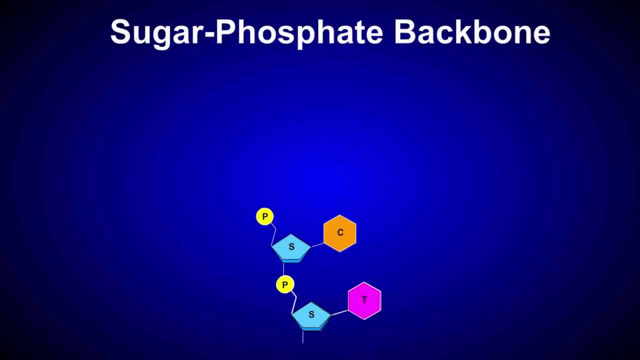 Nucleotides are linked together by dehydration, synthesis or polymerization reactions between the sugar of one nucleotide and another nucleotide. In the process, a sugar-phosphate backbone is formed linking the nucleotides together. Notice how the nitrogenous bases project to one side of the backbone. 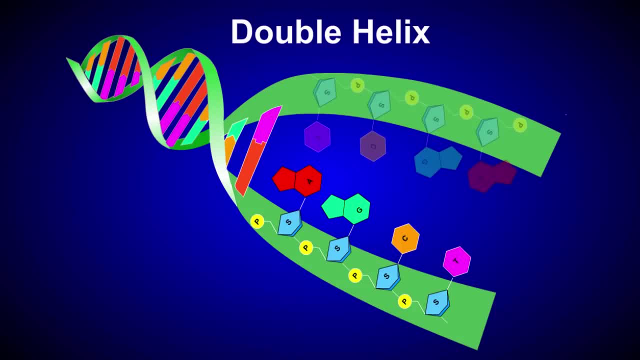 DNA is composed of two strands, arranged as a right-handed helix. The strands are also antiparallel, meaning that they are oriented in opposite directions. The two strands are held together by hydrogen bonds. Guanine forms hydrogen bonds with cytosine and adenine bonds with thymine. 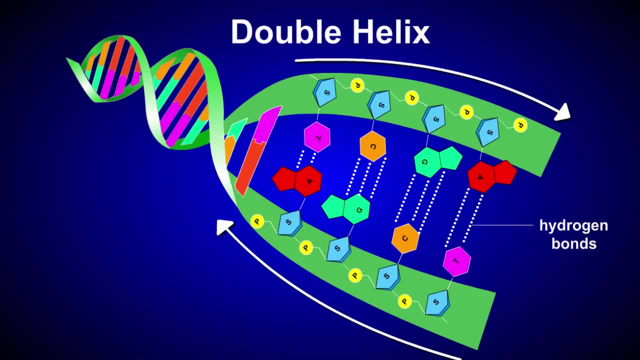 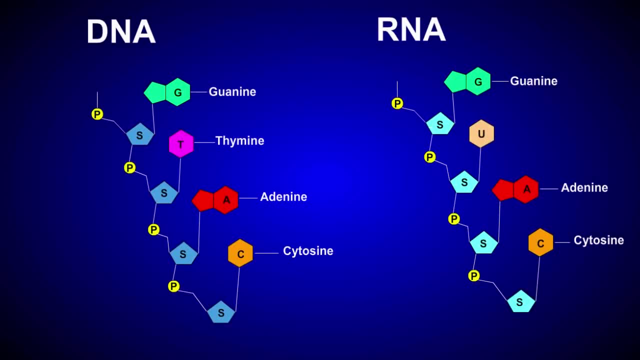 This complementary base pairing links the strands together. It also plays an important role in the replication of the DNA molecule. RNA differs from DNA in that it contains the sugar ribose instead of deoxyribose and the nitrogenous base uracil instead of thymine. 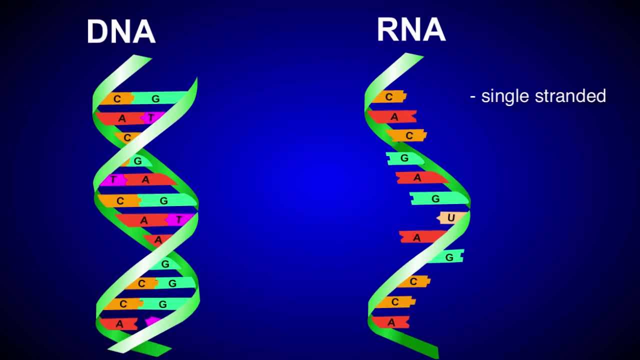 Also, RNA is usually single-stranded and does not typically form a helix. Because of this, it is less stable than DNA and is usually more temporary. While DNA stores the information that is needed to construct a protein, RNA functions in regulating the expression of this information in the protein synthesis process.